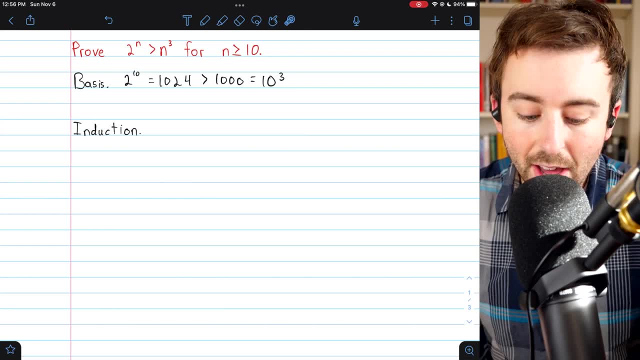 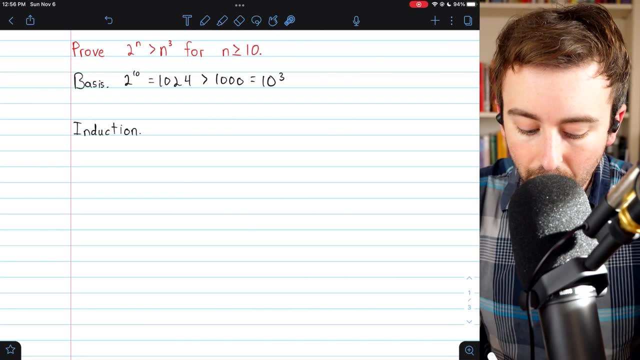 is greater than 10 to the power of 3.. Thus we have shown our result is true for the first number of interest, where n equals 10.. Now we can move on to the induction step. So here is our induction hypothesis. 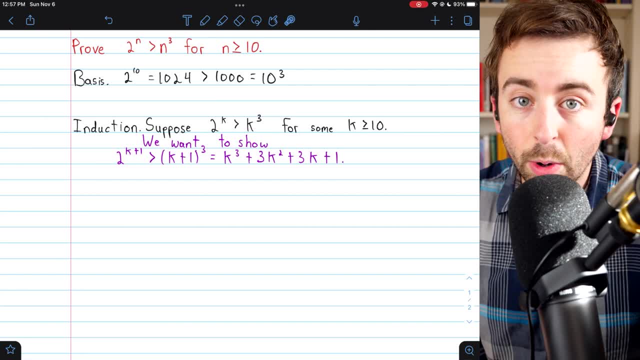 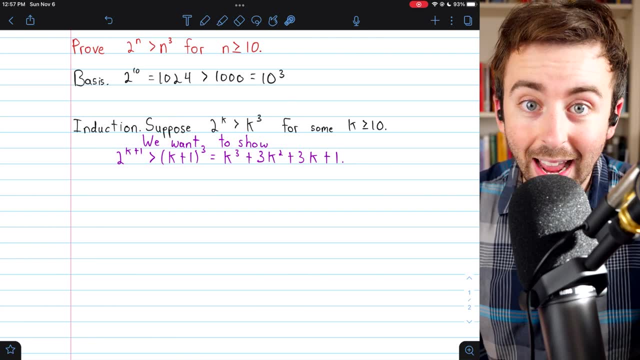 We're supposing that our result is true, so 2 to the k is greater than k cubed for some k, at least 10.. We just proved that our result is true for 10, so certainly we can assume it's true for some value, at least 10.. 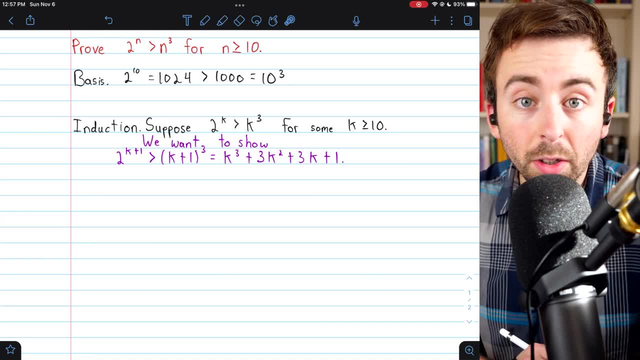 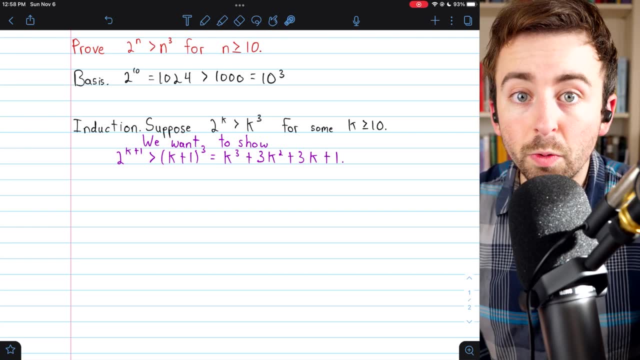 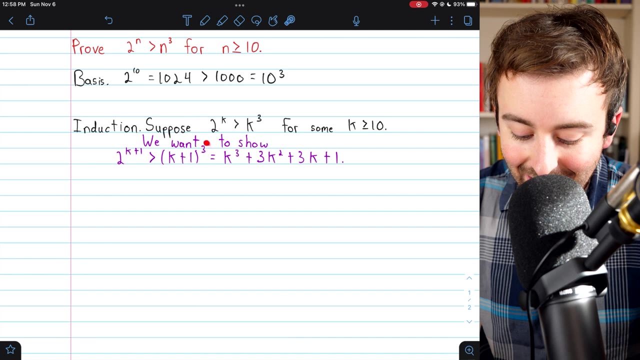 Now, with that said, what we want to show is that our result holds true for the next positive integer. We're assuming it's true for positive integer k. We want to prove it's true for the next positive integer. So we want to show that 2 to the k plus 1 is greater than the cube of k plus 1.. 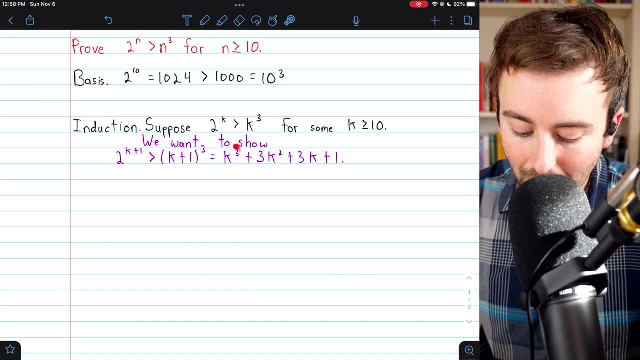 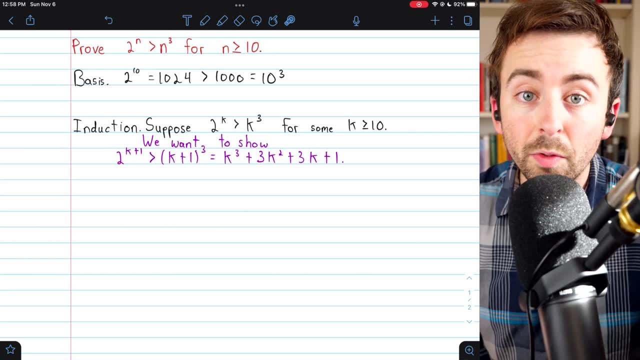 k plus 1 cubed, of course, is equal to k cubed plus all of this if you expand it, And this expansion of k plus 1 cubed is going to be vital for our proof. All right, so to get into this, this is what we want to show. 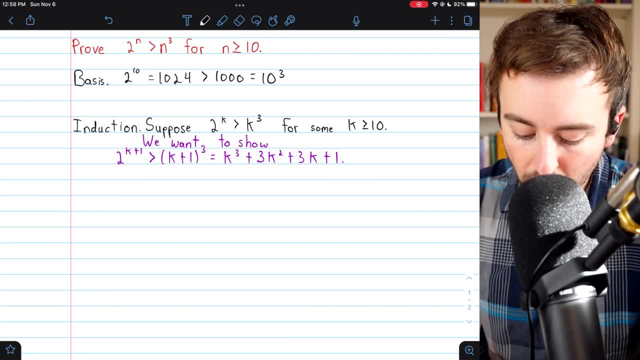 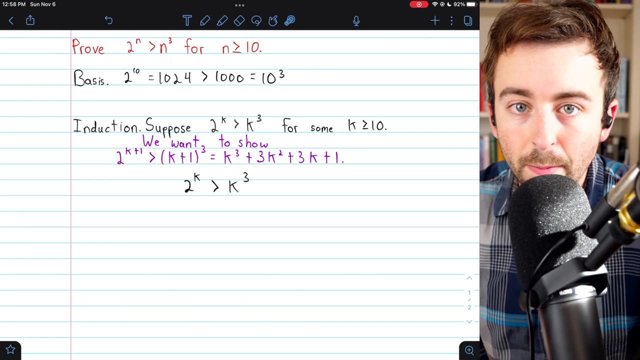 but certainly we can't start there. We need to start with what we know, which is from our induction hypothesis. We know that 2 to the k is greater than k cubed. Now to take a step towards our goal. our goal concerns 2 to the k plus 1,. 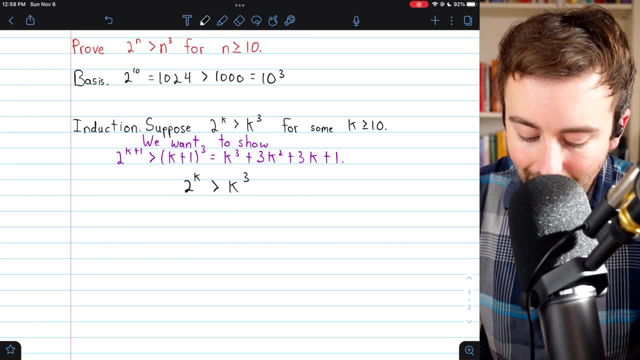 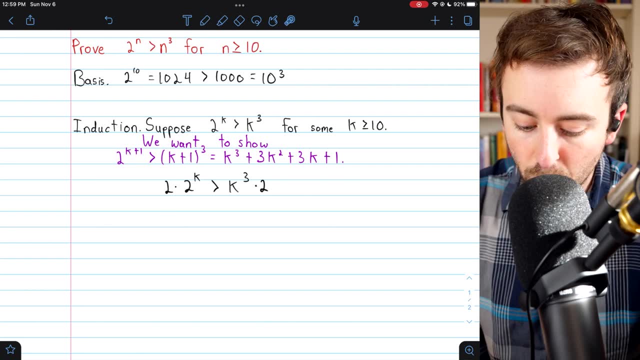 we should multiply both sides of this inequality by 2, because if we do that then we'll have 2 to the k plus 1 on the left, since 2 times 2 to the k is 2 to the k plus 1.. 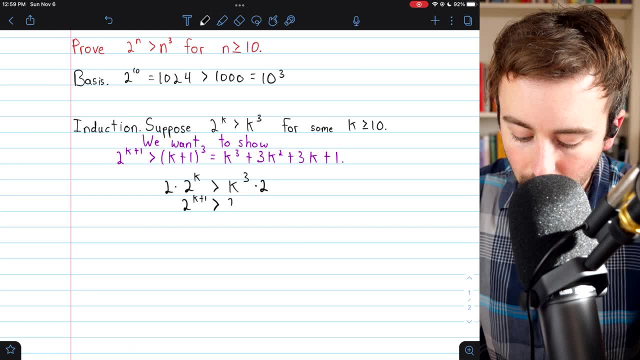 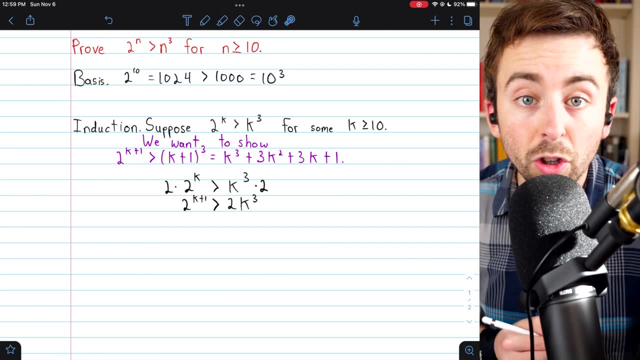 So this gives us that 2 to the k plus 1 is greater than 2 k cubed Again. we've just multiplied both sides of this inequality by 2. At this point we might feel kind of close to our result. 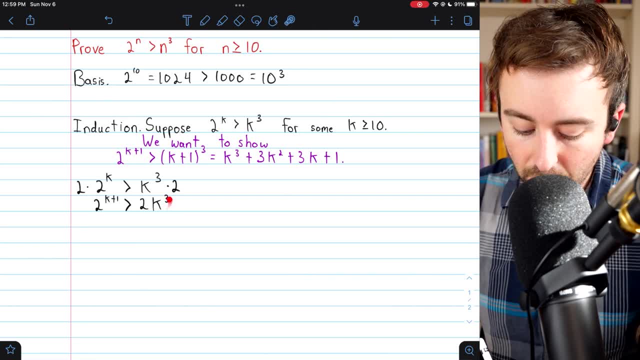 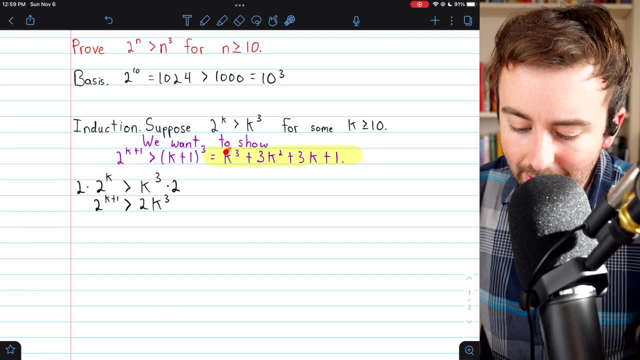 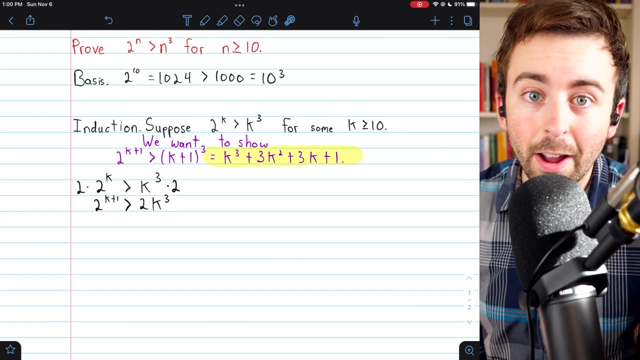 We've shown that 2 to the k plus 1 is greater than 2 k cubed. We're trying to show that it's greater than this. This has 1 k cubed and then a bunch of other stuff, but this other stuff probably isn't as much as an entire additional k cubed, right. 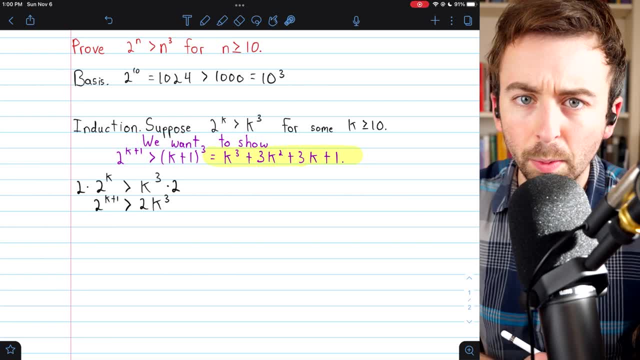 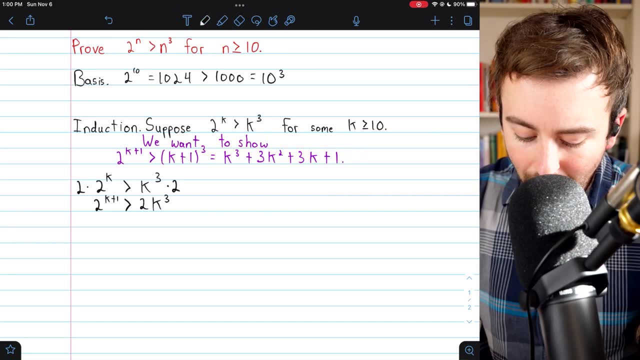 2 to the k plus 1, we know is greater than 2 k cubed. So we're gonna try to leverage that in order to prove the actual inequality that we want. So we're gonna say: well, 2 k cubed, that's the same as k cubed plus k cubed. 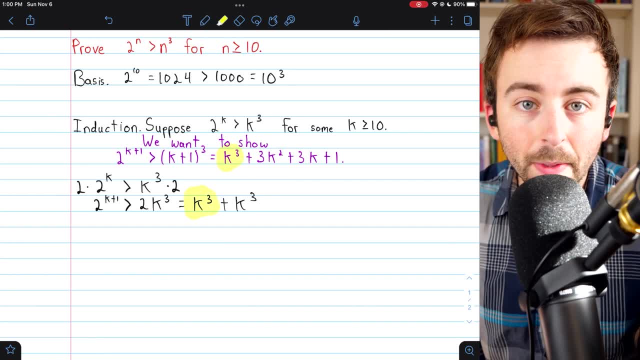 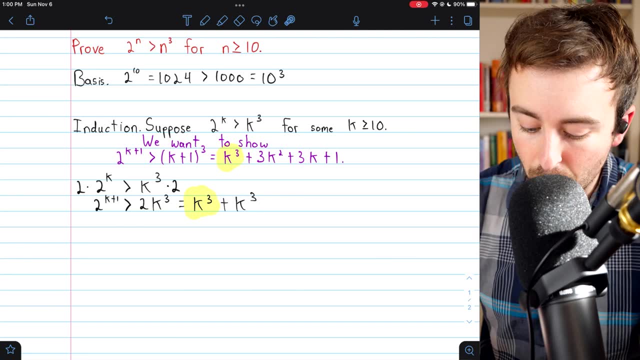 Now this k cubed matches up with this one in what we're trying to prove and this other k cubed. maybe we can show that this k cubed is at least as big as all of this stuff, If we can do that. 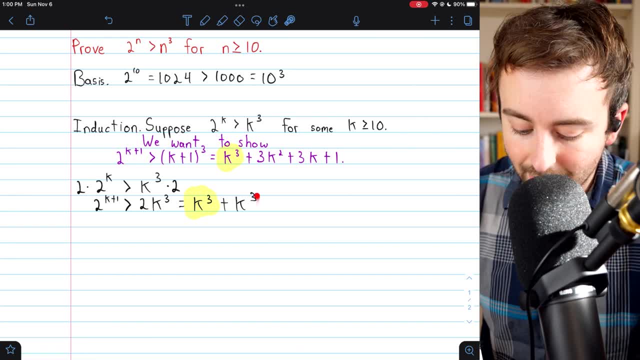 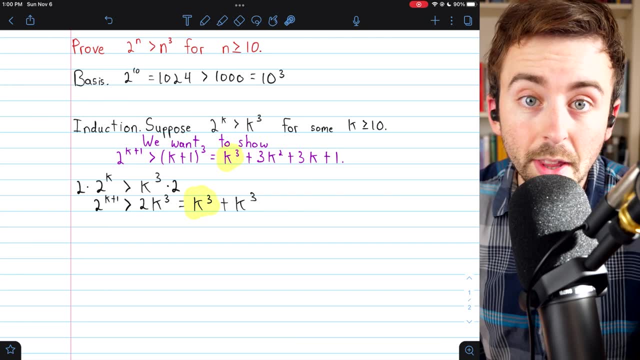 then we will be done, Because then we could replace this k cubed with all of this stuff and we'd have our desired result: that 2 to the k plus 1 is greater than all of this To begin showing. our extra k cubed is in fact at least as big as all of this stuff. 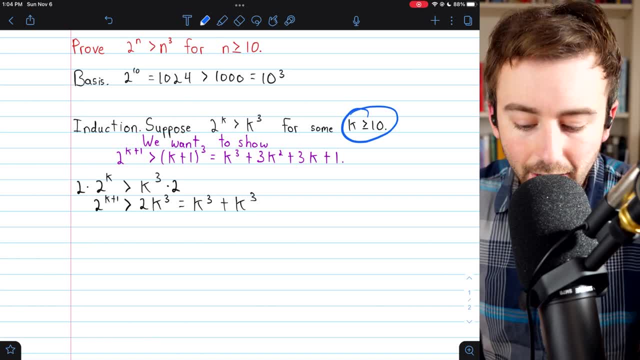 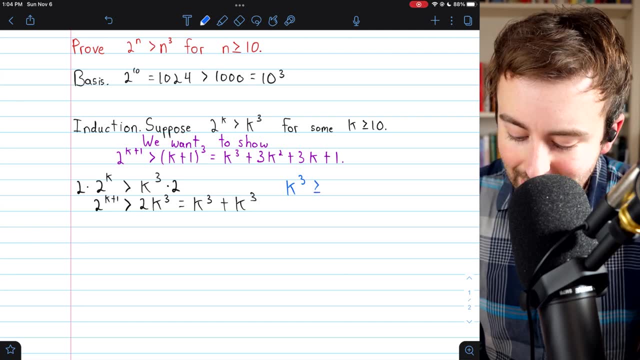 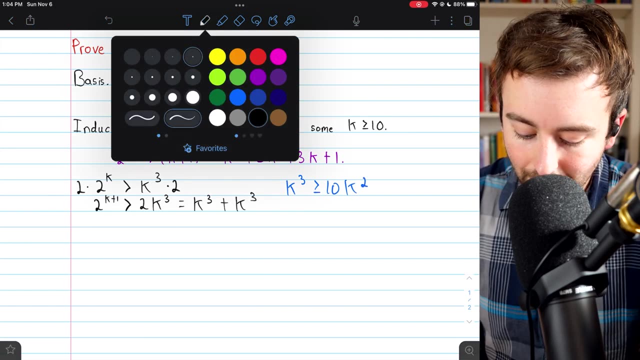 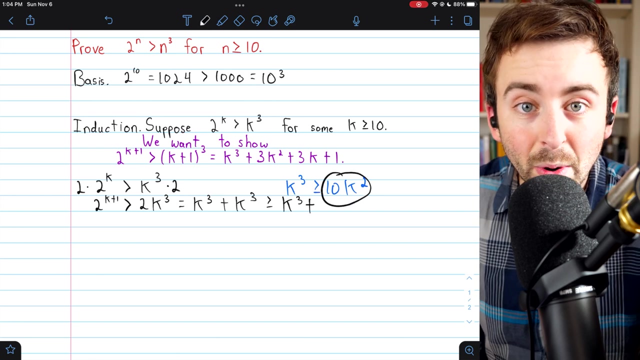 let's recall that k is at least 10.. So k cubed, which is equal to k times k squared, has to be at least 10 k squared Again, because k is at least 10.. So we could say: certainly k cubed plus k cubed is at least k cubed plus 10 k squared. 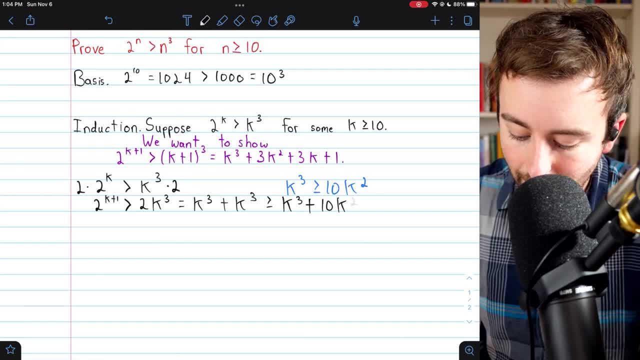 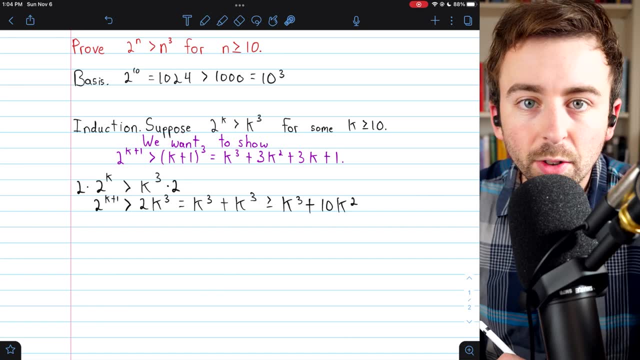 Because k cubed is at least 10 k squared, But the squared term is not the same as the squared term. The squared term that shows up in our expression that we're trying to get to is 3 k squared. So let's take a 3 k squared out of this 10 k squared. 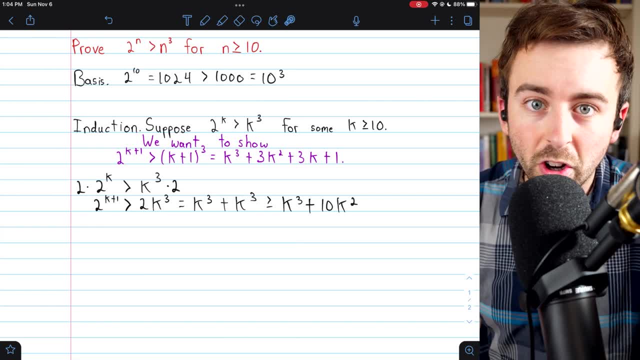 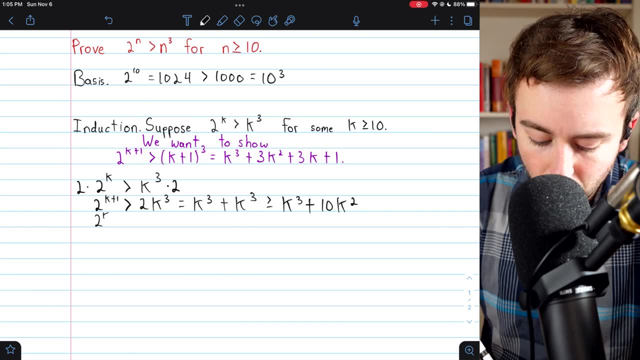 and then we'll have 7 k squared left to work with, And we'll try to show that 7 k squared is greater than the rest of this stuff. So we'll move to a new line and write that 2 to the k plus 1.. 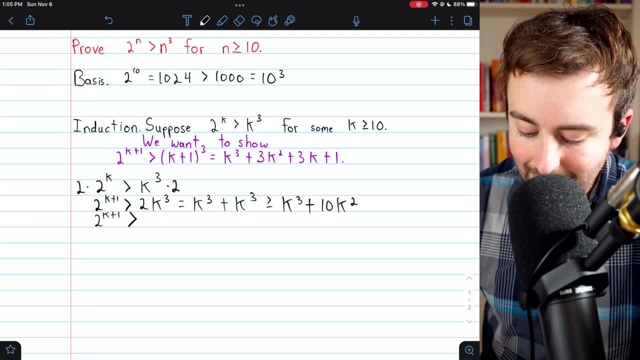 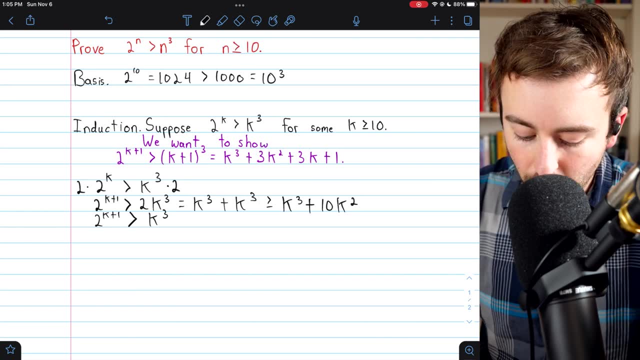 At this point we have that it's greater than k cubed plus and, like I said, we're going to take 3 k squared out of this 10 k squared. So k cubed plus 3 k squared, and then we still have 7 k squared left over. 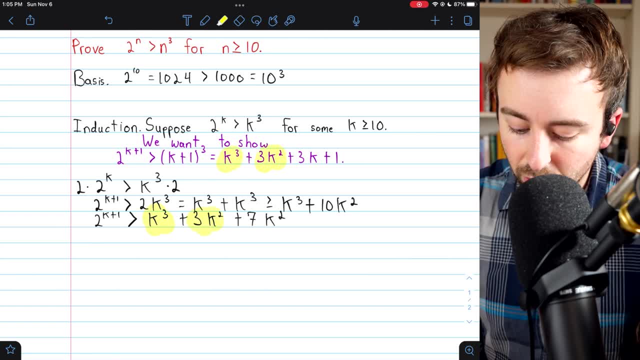 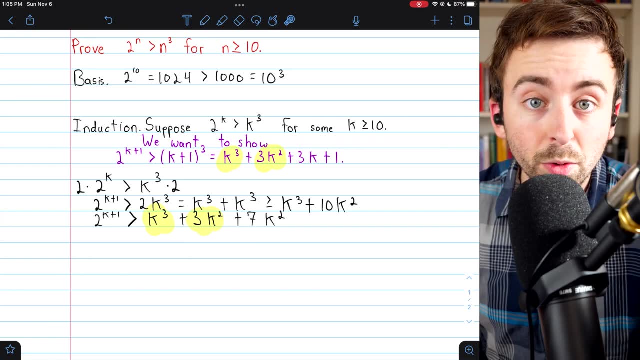 Okay, we've got the k cubed, We've got the 3 k squared. Now we just need to show this: 7 k squared is greater than or equal to 3 k plus 1.. And this is pretty easy because, again, k is at least 10.. 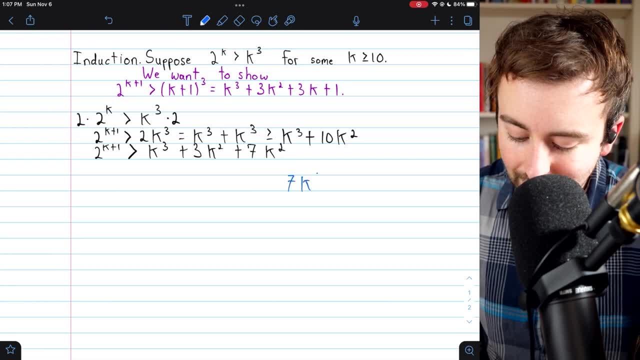 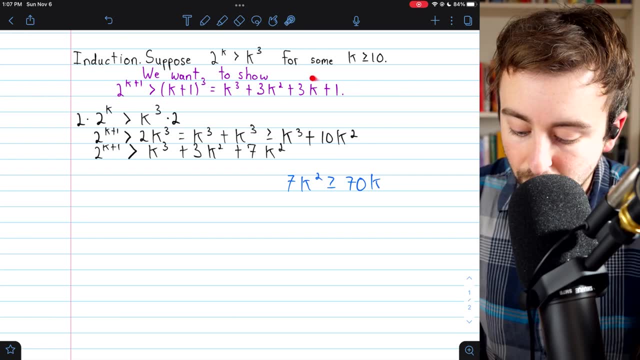 So 7 k squared is is at least 70 times k. So then if we can show that 70 k is greater than 3 k plus 1, will pretty much be done, And that's really easy, because 70 k. 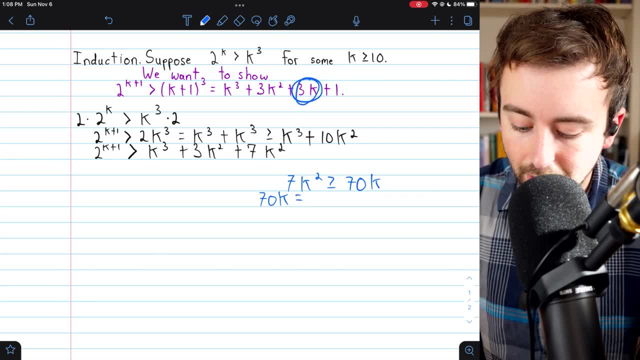 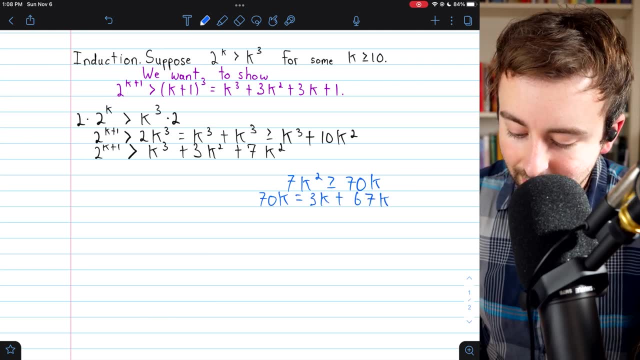 we could split that up into 3 k, since that matches up with this, plus whatever's left over. So 3 k plus 67 k, And then, since k is at least 10,, 67 k, for sure, plus 1.. 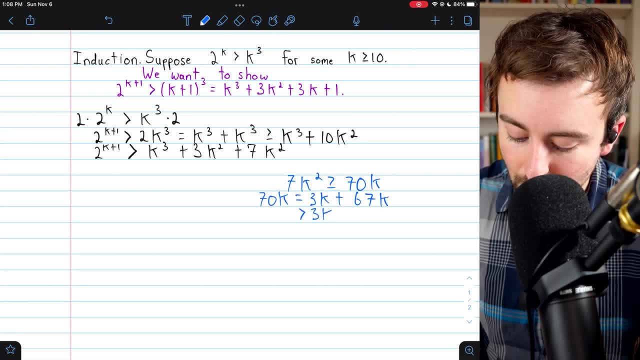 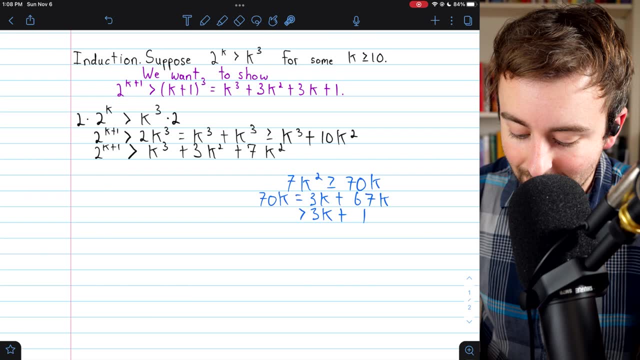 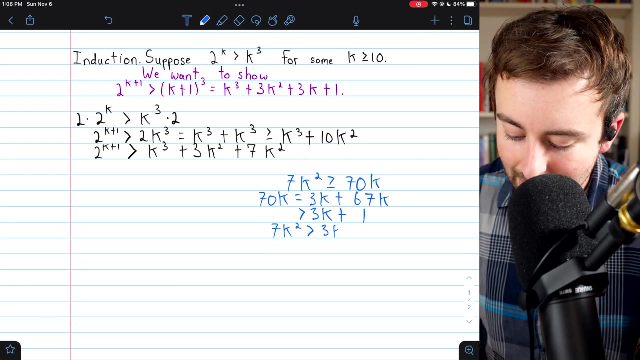 So this final expression here, for sure, is greater than 3 k plus 1.. So 7 k squared is at least this big, and this is greater than 3 k plus 1.. So then we have that 7 k squared is greater than 3 k plus 1,. 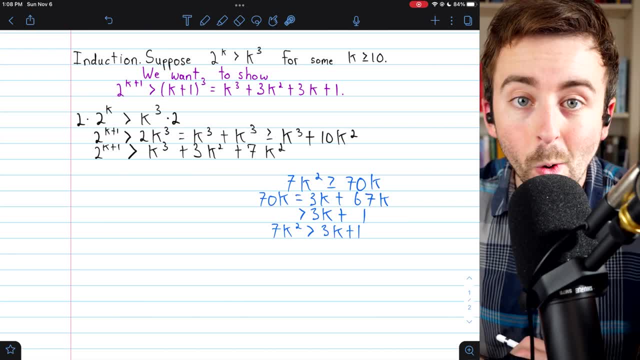 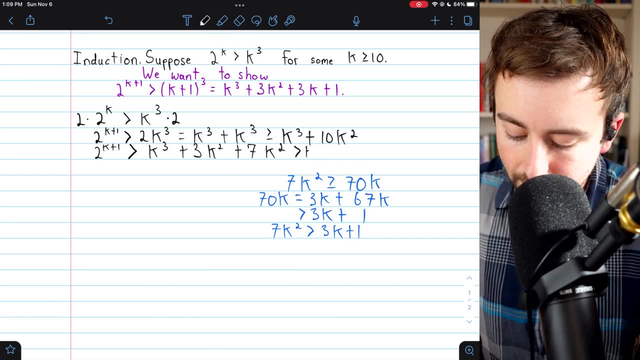 and we can make this final replacement in this inequality: Since 7 k squared is greater than 3 k plus 1, this whole thing is greater than k cubed plus 3 k squared plus 3 k plus 1.. 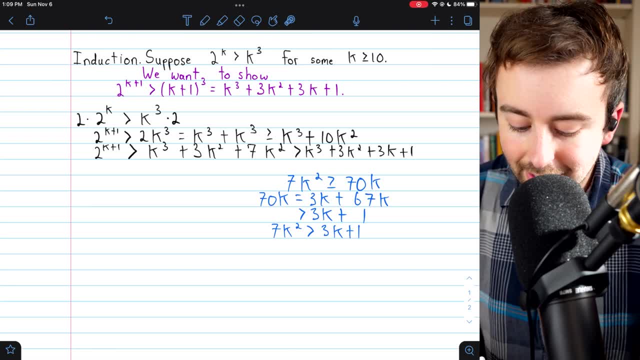 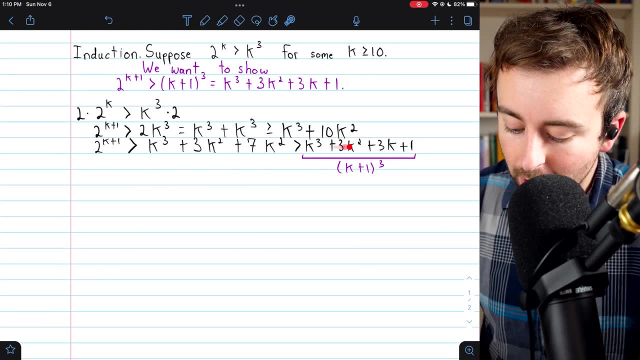 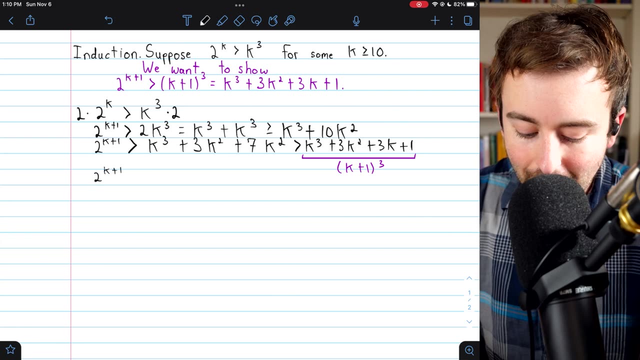 And this whole sum is equal to k plus 1 cubed. So 2 to the k plus 1 is greater than all of this, which is greater than all of this, and this is k plus 1 cubed. So we arrive at our final desired statement here. 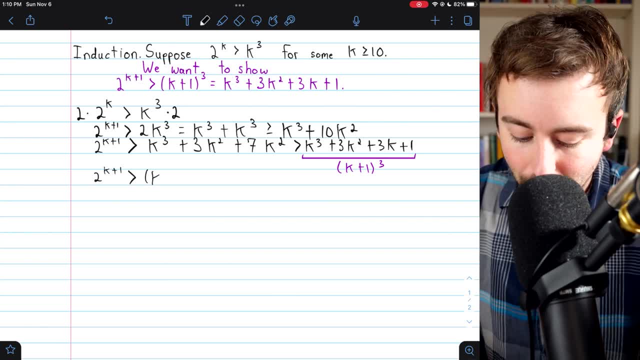 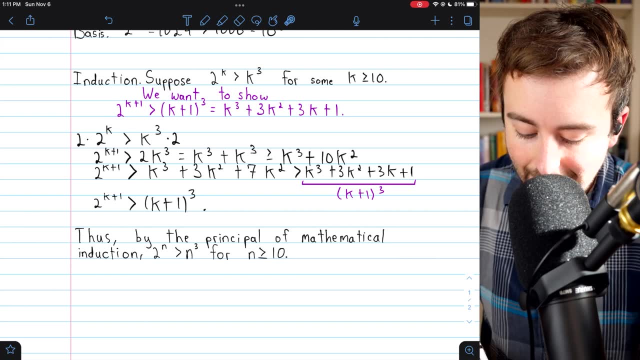 2 to the k plus 1 is greater than k plus 1 cubed, And so we've completed our proof. By the principle of mathematical induction, we've shown that 2 to the n is greater than n cubed for n at least 10.. 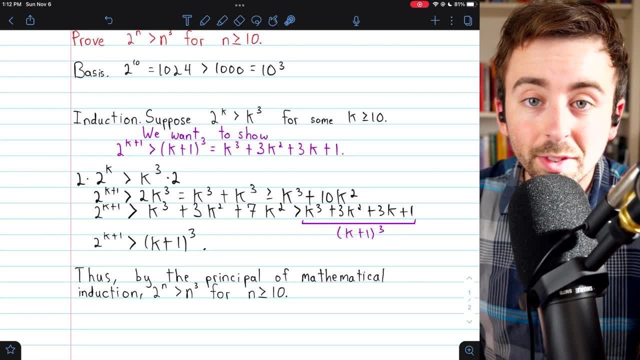 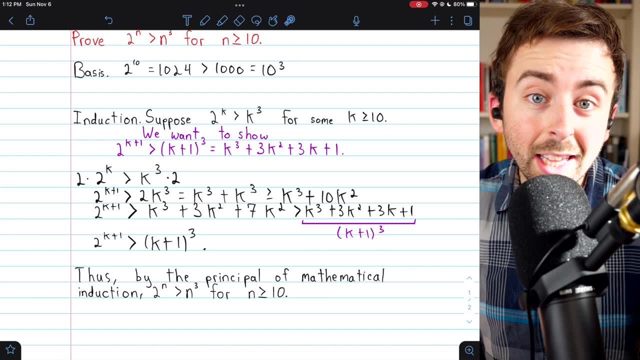 We prove that it's true for the first value- n equals 10, and then show that if it's true for one value, it has to be true for the next. Hope this was helpful. Let me know in the comments if you've got any questions or video requests. Thank you for watching.